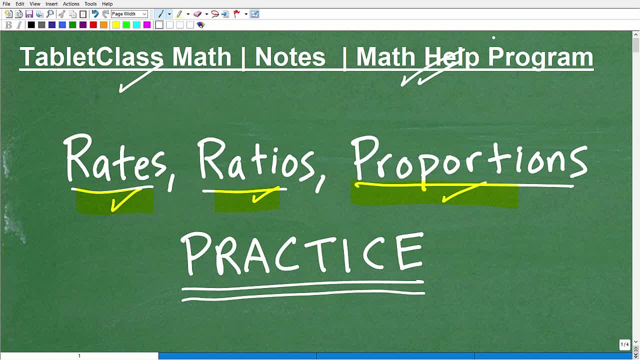 For example, like to get yourself ready for the GED or ASVAB test or college placement exam, teacher certification exams, ACT test. So what I do with all my courses is I do a lot of research on what's going to be on those particular tests And I kind of build custom courses for those demands or for that particular test. So it's a lot of work. It's taken me years to build And if you need math help, 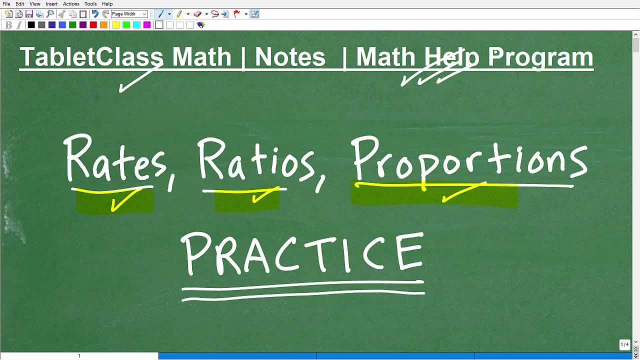 whether you need assistance in a course you're taking. you need to take a full online class or like homeschool. I do it all, So just check out my math help program And you can see the various options there, But I think you'll be very happy with that. if you're looking for math help Now, you know YouTube is a great platform to get assistance, And that's why I make these videos there for you. But you have to do something as well, And if you're a math student, you have to do the following: Okay, you have to take great math notes over. 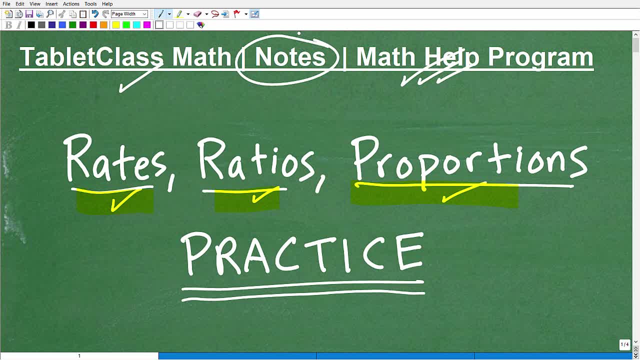 decades of teaching math. There's one thing is apparent to me. I call it my golden rule: math. That is, those students who take the best math notes almost always have the best math grades. And those students who don't take math notes, who think they have some like photographic memory. they could just remember every single thing. They kind of talk themselves into that, like I got that. Now are there people who have photographic memories? Yes, they're like very, very point 0001% of you know human beings out there. I'm not saying there isn't or there isn't. 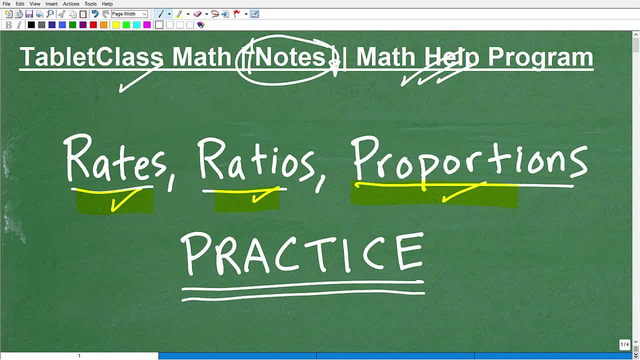 There isn't prodigies and stuff. But listen, even those folks, I'm sure, take notes. you have to take notes, Don't you know? rely on your best friend in the back of the class because they write neater than you. You're like. you know I like your notes better than mine. You know, when you're done with your notes, I'll just copy your notes, you know. whatever the case is, listen, I've done it all. You know, I was a student once And, believe me, when I was at school until I really got serious in my math degree program. you know, I've done it all. 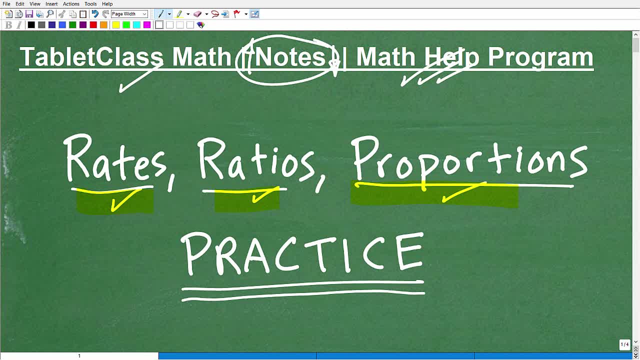 And I found out pretty quick the consequences of not taking great math notes. So, listen, do the work. okay, and really work on your note taking. it's going to pay off big time. Okay, But it's not optional, right? You got to really, really work hard at taking great math notes. So improve. if you need to improve- And most of us, all of us- can- you know there is room for improvement. But in the meantime you need something to study from. So I have detailed, comprehensive math notes to include pre algebra, algebra one, geometry, algebra two and algebra three. 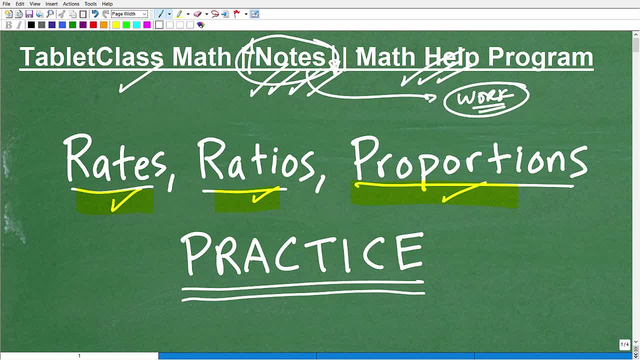 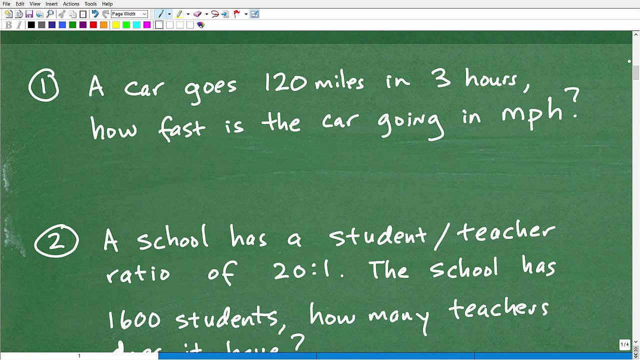 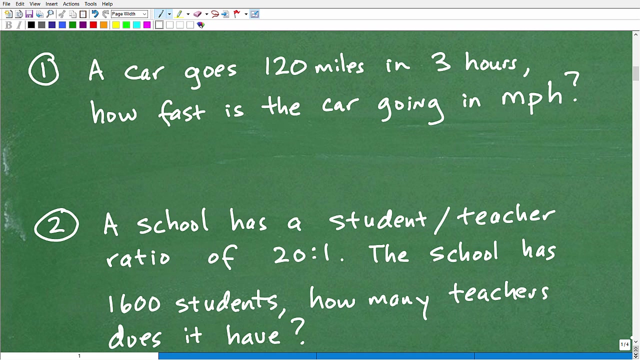 And trigonometry. you can find links to those notes in the description of this video. Okay, now let's get into rates, ratios and proportions. Let's take a look at our practice problems here And then I'm going to go over each one, but I'll give you a chance to solve this if you kind of want to use this as a little quiz. So again, if you're not, you know, if you're don't know how to do these problems, you just go back to some of my other videos on these topics to kind of learn about it And you can come back. 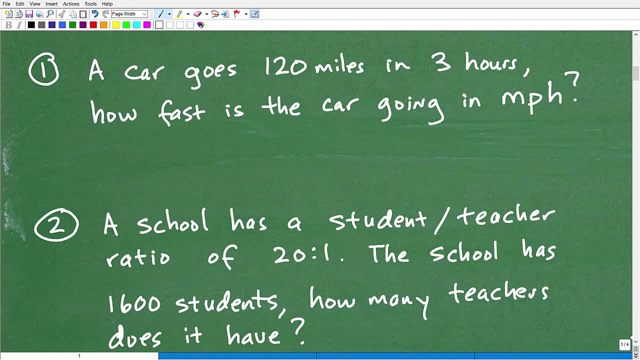 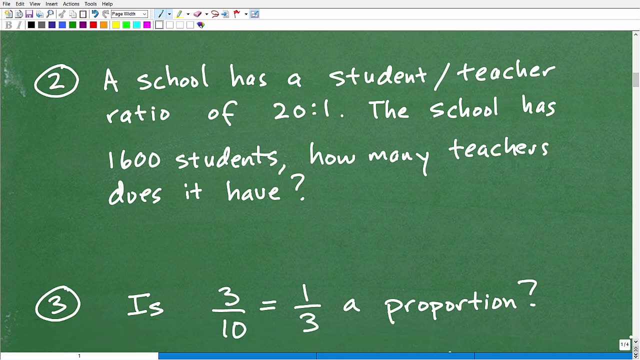 to this video. So here is our first problem: A car goes 120 miles in three hours. How fast is the car going in miles per hour? Okay, so that's our first question. Our second question: Okay, of course you can pause the video or rewind it to see these questions one by one. Our second question is: a school has a student teacher ratio of 20 to one. The school has 1600 students. How many teachers does it have? Okay, so that is our second question. 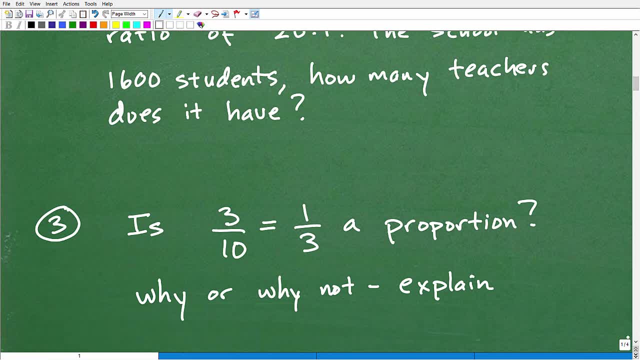 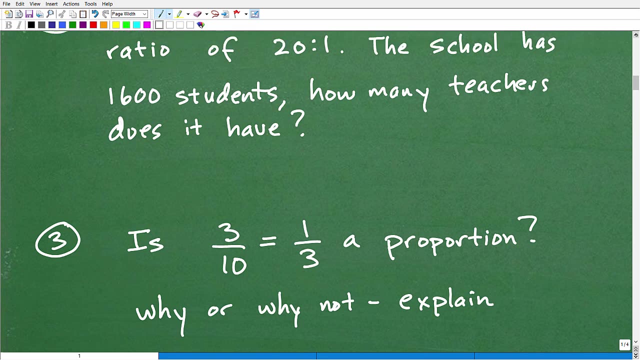 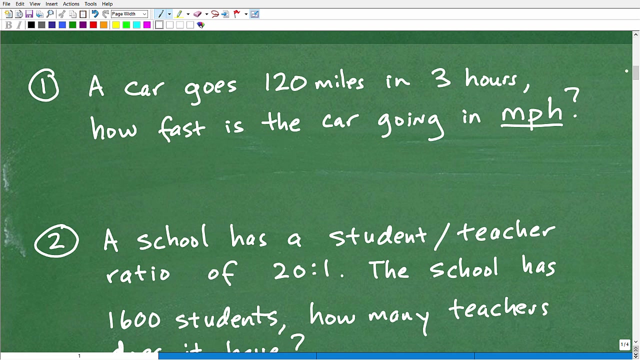 And then our last question we'll be doing here in this practice problem set is: three over 10 equaling to one third, or three tenths equal to one third a proportion. Okay, please explain why or why not justify your answer. That is our three questions. So again, let's go back to question number one. If you want to pause the video and work through these, or if you just want to see me solve these problems, just continue to watch the video, because I'm going to do this right now. 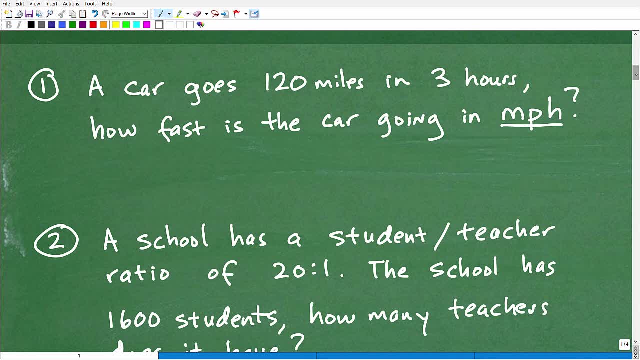 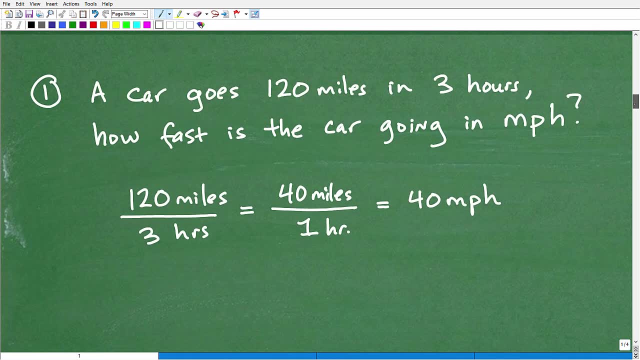 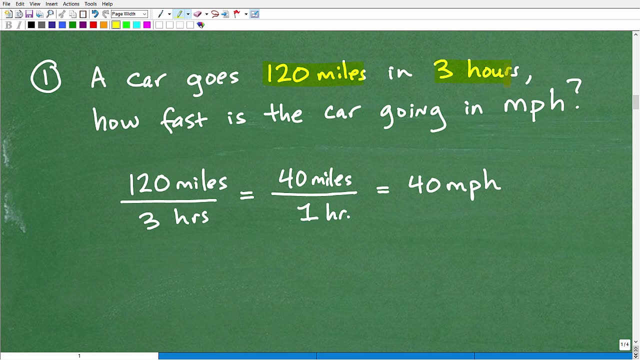 Again, if you don't want to see the solutions and you want to work on these problems, pause the video rewind, etc. Because I'm going to get into the solutions right now. Okay, so here we go. Number one: a car goes 120 miles in three hours. How fast is the car going in miles per hour? So this is an example of a rate. Okay, a rate. Now I got the word here, the solution here, but let's just talk about a rate. 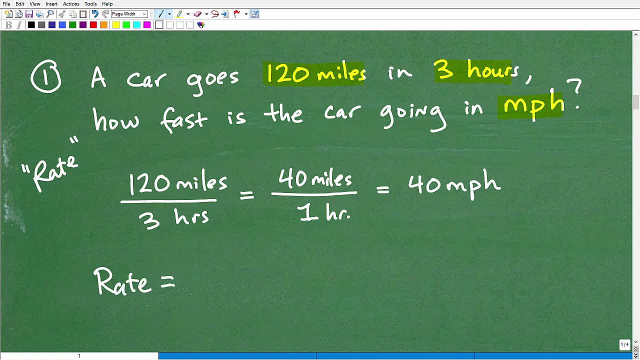 All right, this word rate is oftentimes, you know, synonymous with speed, the speed of something or the velocity of something. Okay, so if you're thinking like a car is going- you know I didn't use the word rate in the question here- But if you're thinking about, is this a rate or a ratio, Well, it's a rate, Okay, because we're talking about what's the rate of the car, What's the speed of the car. But what is the definition of a rate or a ratio? 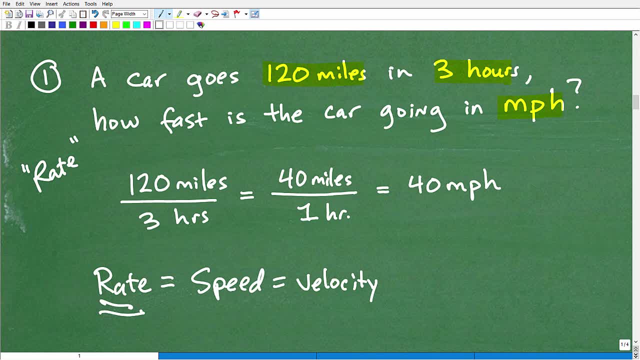 Okay, well, I'm going to go ahead and just review this right now. Rates, ratios and proportions are all fractions. We're talking about fractions. we're comparing two numbers. In this case, we're comparing 120 miles and three hours, And we're going to do that as a fraction. So this car is going 120 miles, And then this fraction bar, who would say the word per? okay, it's going 120 miles per three hours. Now, what makes this a 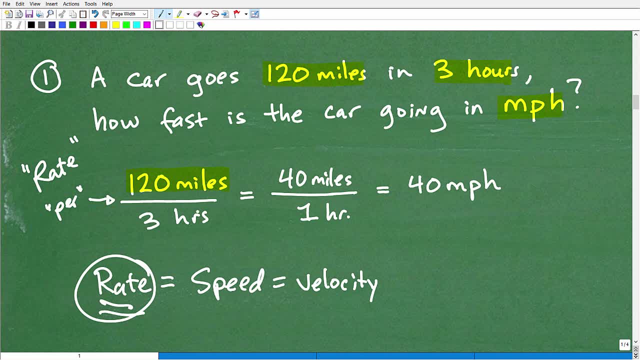 rate and not a ratio is the units of measure. Okay, we have to really focus in on the units of measure here. We're comparing distance- miles- and time. we're comparing two different units of measure: distance, okay, and time, right, Anytime. you're comparing two different units of measure in a fraction, that is a rate, Okay. so miles per hour is a. 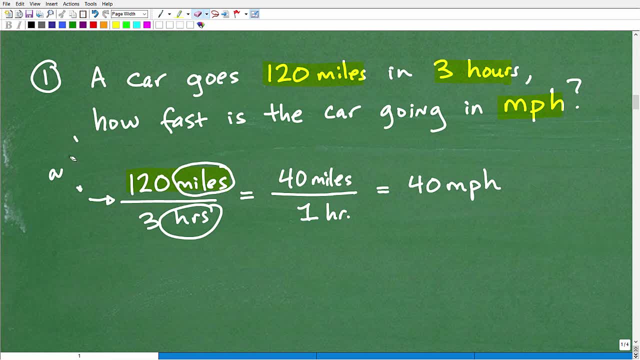 unit of measure of a rate, Okay. so let's just kind of erase all this. But that's what this is. Again, we're practicing these concepts. just a quick review. But you know, these little problem, this little problem here, is not a subsidy for you learning more about rates, ratios and proportions. But if you didn't know anything, now you know. okay. so, 120 miles per three hours- this is the way I can express this as a rate. But I want to know miles per hour. Okay, so that means I want to get what we call. 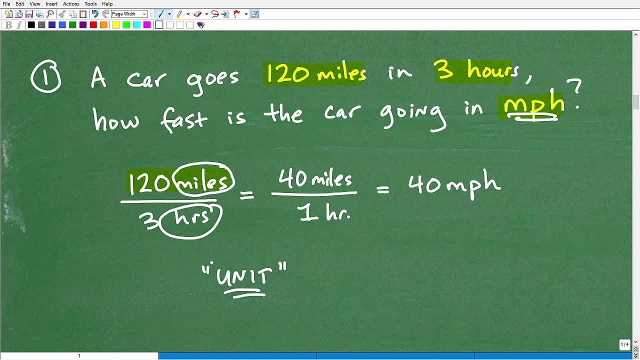 unit, the unit rate, okay. sometimes you're asked to find the unit rate or ratio, and that's when the denominator is equal to one. so if i simplify, 120 over three, now reduce that fraction, that's 40 over one. okay, because three goes into 120, uh, 40.. so this is 40 miles per one hour, or 40 miles. 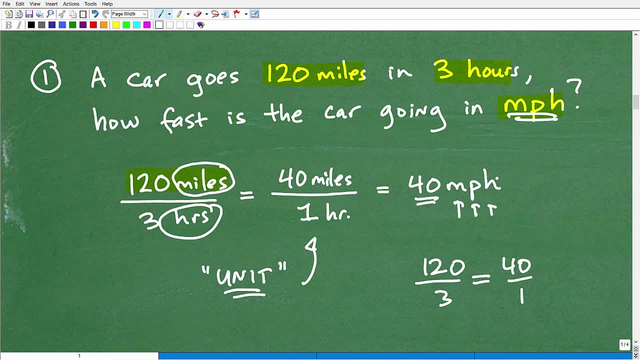 per hour because it's one hour. okay, so that's the miles per hour. so how fast is this car going in miles per hour? it's going 40 miles per hour. now, if you kind of just, you know, divided 120 by three and you got 40, and like at 40 miles per hour, yeah, that's good, okay, uh, but do, were you in? 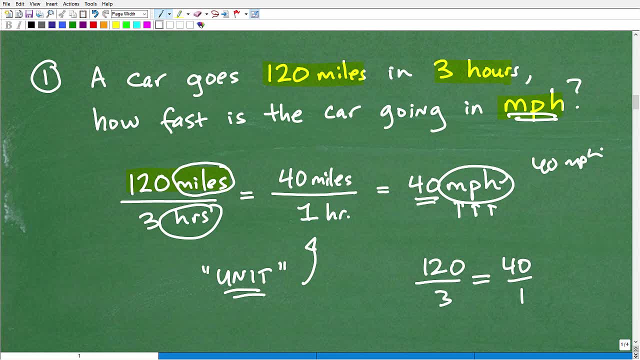 command of the concepts. can you fully explain? could you teach this to your little brother or sister and be like, listen, here i'm going to teach you how to do rates. da, da, da da when you? this is a good, uh way to know if you know something, if you can teach something in a 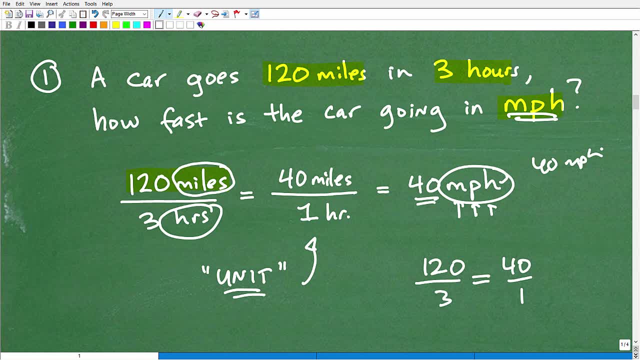 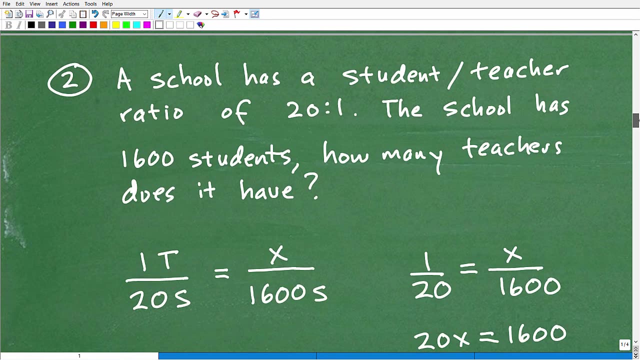 really concrete way, like in a complete way, that means you really have learned it. okay, that's a very, very good indicator, uh, to uh see if you really understand something is if you can teach it, all right. so let's move on to our second problem, and uh, of course, this is about everyone's. 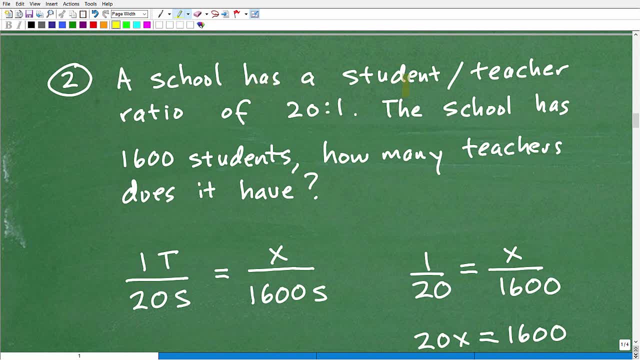 favorite topic: school. so we have a school has a student teacher ratio- and of course i'm using the word specifically here- ratio of 20 to 1.. now this little notation here: 20 to 1, i could say 20 to 1, but this uh colon there, like that, is a very common way to express. 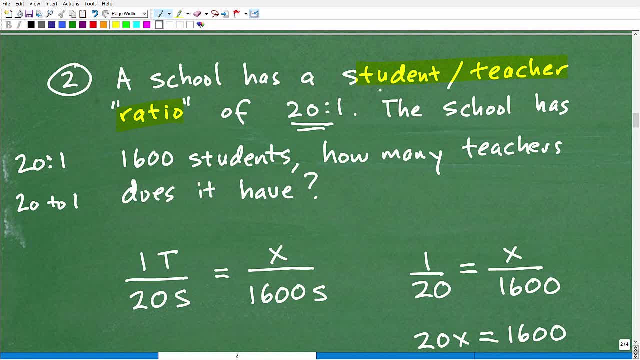 ratios 20 to 1, and this description is very common as well. so you know, there's in a classroom there'll be 20 students and one teacher, so this is a very common way to express ratios 20 to 1 and this. so that's kind of like the uh policy of the school. hey look, we're going to have- um, you know, for every. 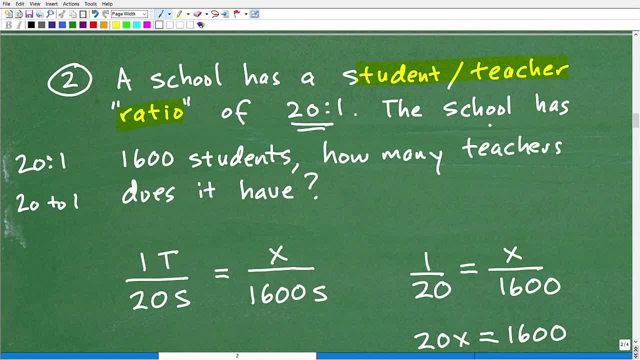 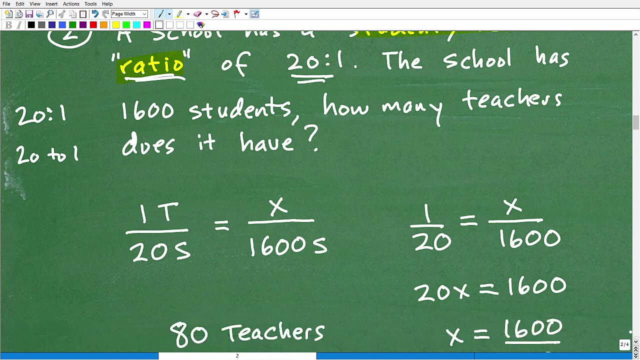 20 students, there'll be one teacher, okay. so the question is: the school has 1600 students total. how many teachers does it have to? uh, obviously be in alignment with this 20 to 1 ratio and of course i'm being told it's a ratio. now let's take a look at uh this here, because sometimes there's 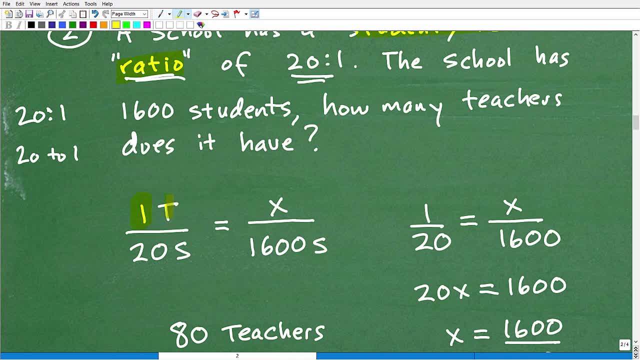 some confusion. so 20 to 1 student teacher ratio: one teacher for every 20 students. now, some of you might be like: aren't these units different teachers and students? you're like: no, they're not, because what are we counting here? okay, we're counting human beings, we're counting people. now, some of you out there were like: well, 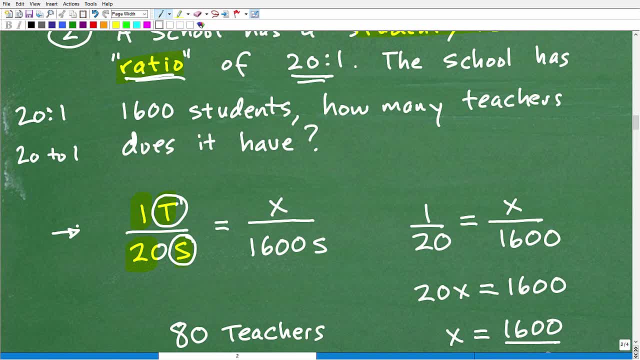 teachers are not really human beings. they don't count. listen, i'm being kind of funny, of course. no, teachers are people too. uh, even math teachers. uh, we are human beings. so we're talking about people, right, we're counting people in the numerator. we're counting people. 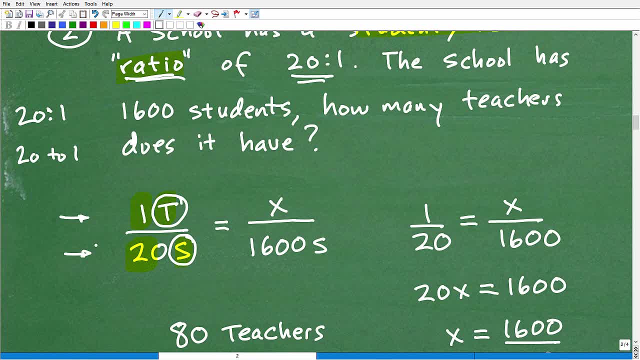 in the denominator all right, whereas a rate, we're counting miles, distance, which is completely different than the concept of time. so that is a ratio, ratios when you're comparing, uh, two values in a fraction and the units of measure. um, what you're counting conceptually? the units of measure. 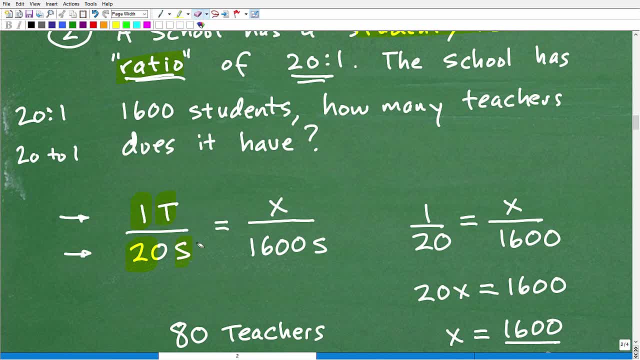 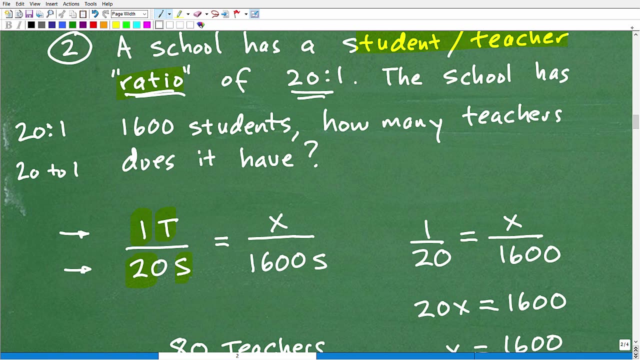 are the same. okay, all right so, but again it can be a little confusing because teachers and students seem to be different units, but they're not okay. so what we're going to do here is we're going to set up a proportion to solve this problem. okay, and a proportion is, uh, two equal fractions. so i have one teacher is equal as um one teacher. 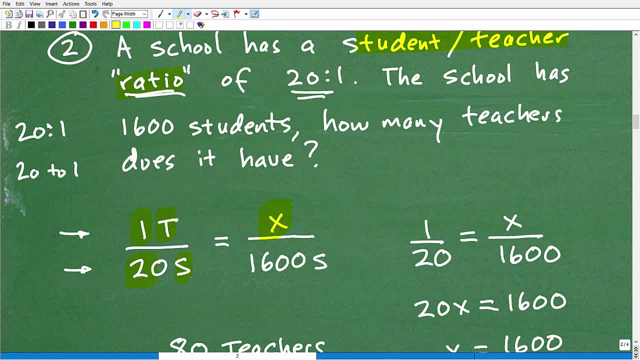 to 20 students is the same as how many teachers? okay, i don't know how many teachers, it's x amount. that's what i'm trying to solve. uh, to 1600 students. okay, so, whatever, this fraction is okay, this fraction. when i get the right number of teachers, all right, this would reduce down. 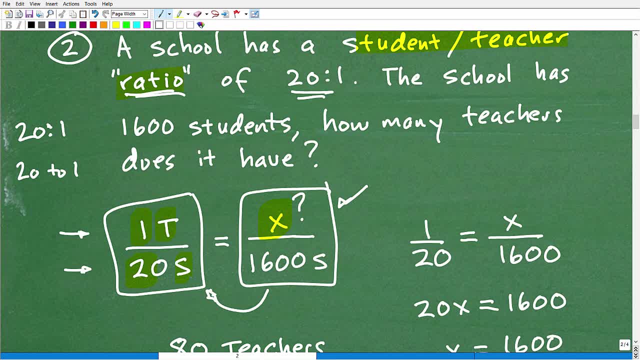 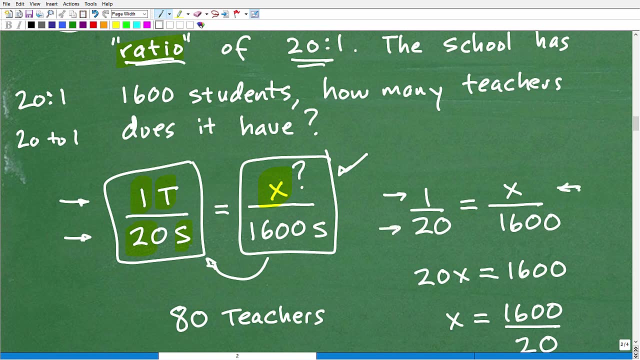 to this right here: 1 over 20. okay, the unit ratio. well, it's not technically the unit ratio because one's not a denominator, but you get the idea. okay, so this is a proportion. this is how you set up this problem. so again, one teacher to 20 students. how many teachers to 1600 students? all right, well, 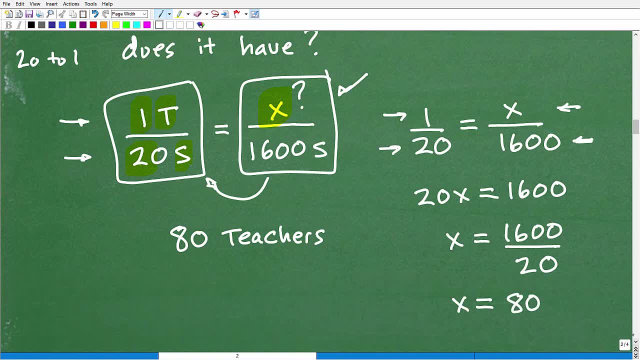 how do i solve this problem? well, you got to know a little bit about proportions, and this is what we call. the means are equal to the extremes, but i like to just use what we the good old-fashioned cross product. so we could just cross, multiply to solve this proportion, all right. so 1600 times 1 is 1600. 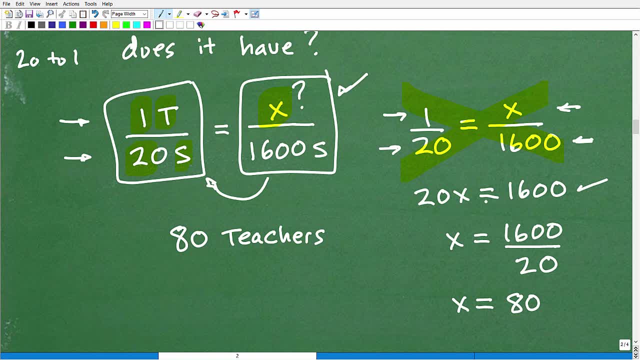 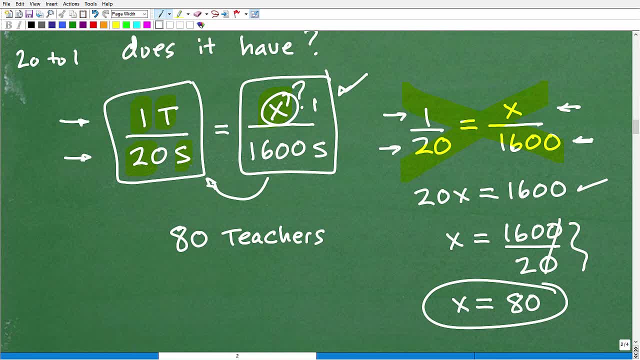 equal to 80. and what does x represent? well, this was the amount of teachers that i need to have, that 20 uh. 1 to 20 student teacher ratio. so x is uh represents 80 or 80 teachers. okay, so with our student population of 1600 and a student teacher ratio 1 to 20, you're going to need to have 80. 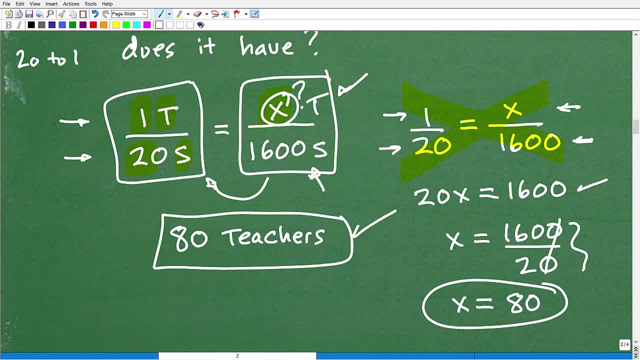 teachers okay. so if you got these problems right so far, definitely give yourself a smiley face and keep that smiley face and i'll see you in the next video. bye, bye going if you didn't get these problems right, but you're understanding right, so that's good stuff. 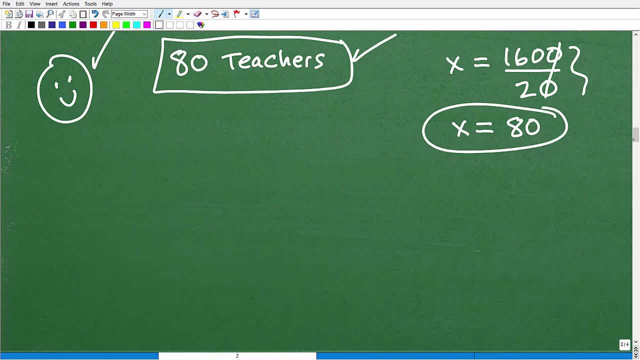 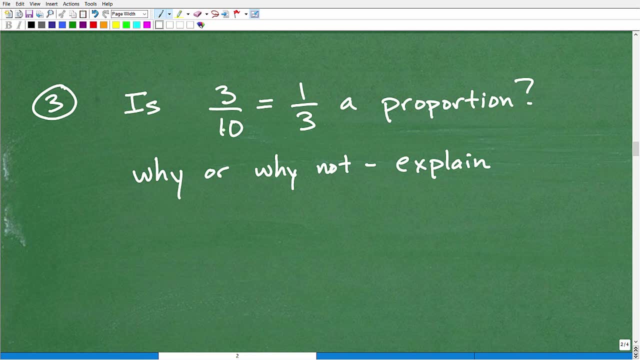 let's move on to our last problem. and this last problem should be easy now, because i kind of gave the answer away and, uh, let's go ahead and read the problem. so is three tenths, uh, equal to one third a proportion? now, if you've been paying attention, you should be able to confidently 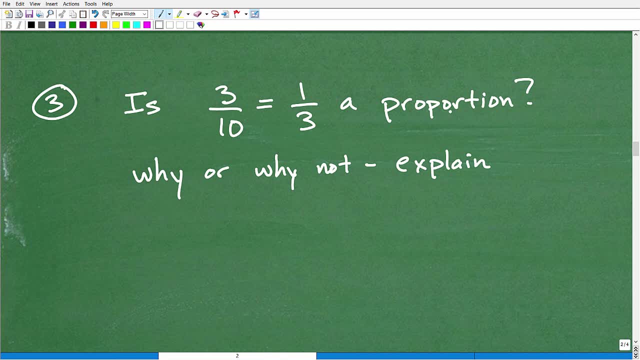 answer this question, okay. so what do you think? yes or or no? the answer is no. okay now, why not okay? well, we got to explain that to you in the next video, bye bye. so why not? well, because if you have a valor proportion, when- uh, basically what that means. 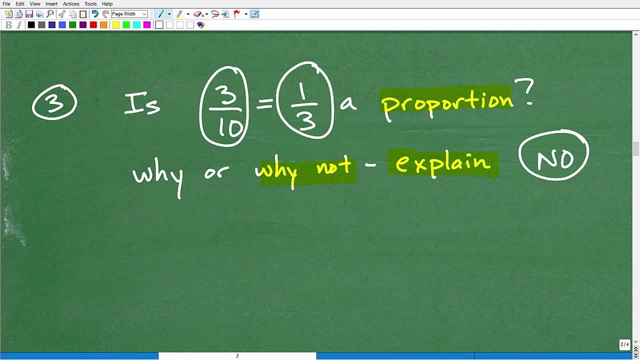 is that you have a fraction that's equal to another fraction. so you might be able to just see here that these are not, uh, two equal fractions. okay, you're like well, but how can we, how can we, um, absolutely uh, explain this? you know 100 kind of way, like hey, i'm going to give you complete. 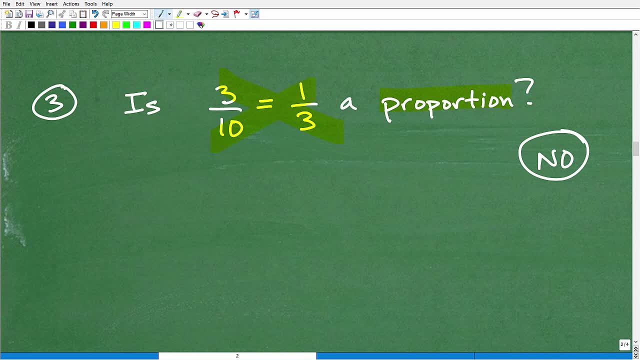 justification right now. well, the way you would do that is to say that you have a fraction that's equal to another fraction. okay, i'm going to give you complete justification right now, though didn't you know that that's true? okay, let's just pause right now andそして. 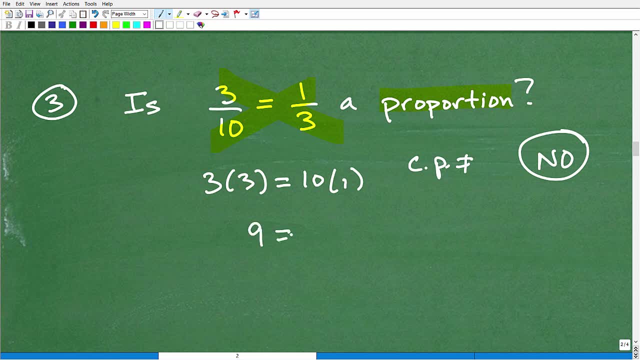 let's, uh, understand this. something is actually lined up that's weird. and then this is really trying to think of all the different equations we need to know, okay, so here's the thing here, if we are, when we read the equation, we use the actual ever investing values and the information. 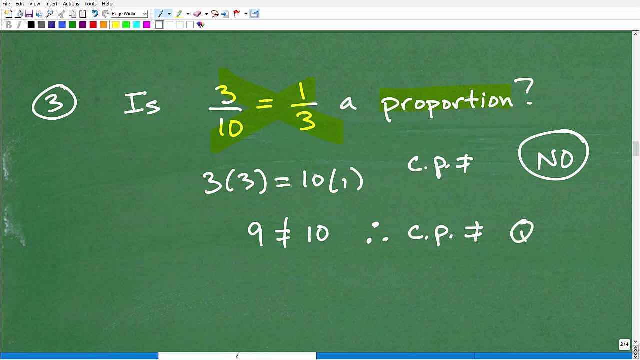 that we share is the average margin. okay, so that's, as example, the average. what would be the 설�icinc Q-E-D? If you really want to learn something crazy about mathematics, look up the word Q-E-D, It's a Latin phrase. 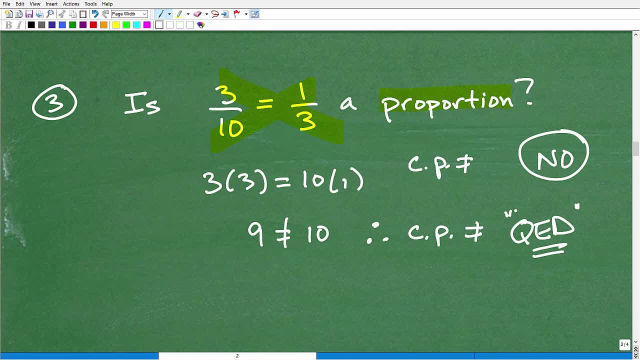 basically, as demonstrated as A big part of studying very advanced mathematics For me- I have a degree in mathematics, theoretical mathematics- We really focus in on proving things, showing if something's true or not true. It's all about justification. We've got to justify. 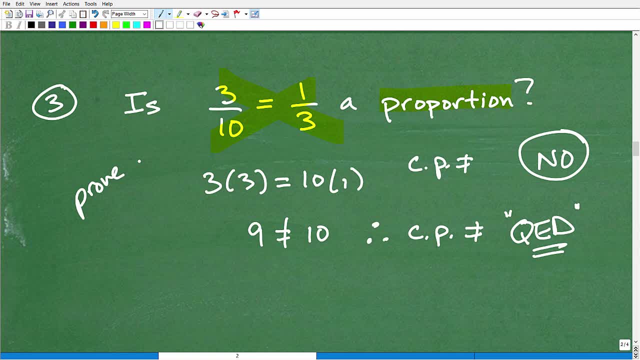 our answer and give reasons, as you do. That's why you need to show your work. The only way you can show your work is if you've been practicing this stuff correctly. The only way you can be practicing this stuff correctly is if you've been taking great notes and paying attention. 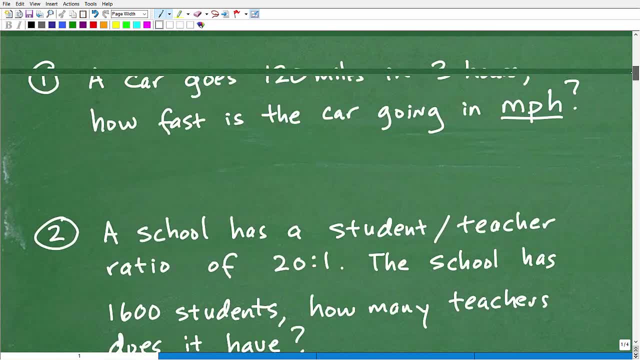 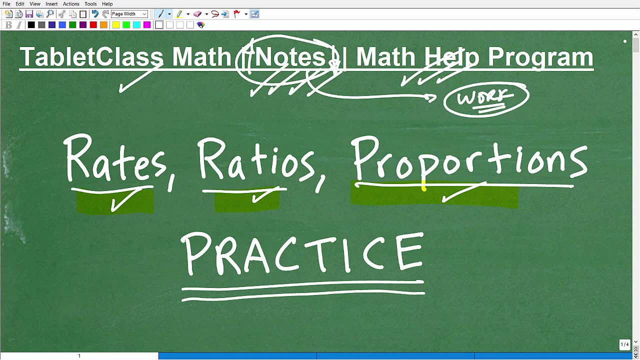 Quick practice on rates, ratios and proportions. If you did well on this topic, does that mean you're a total expert? No, it means definitely you're on the right track. You could be Outstanding in this topic right now, but it's a worthy topic. 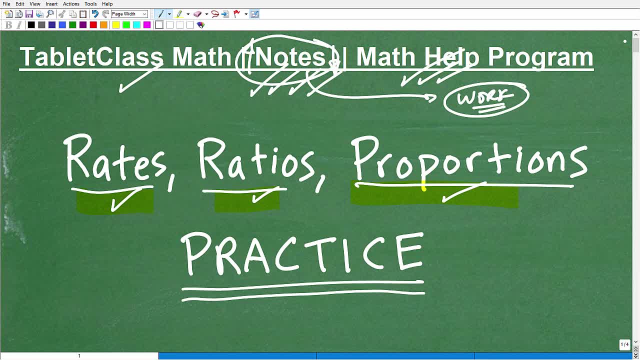 It's an important topic for you to practice. If you ace this quiz, definitely give yourself a gigantic smiley face, an A+ and a 1,000%- That is impressive. That means you're doing well in math. but you've got to. 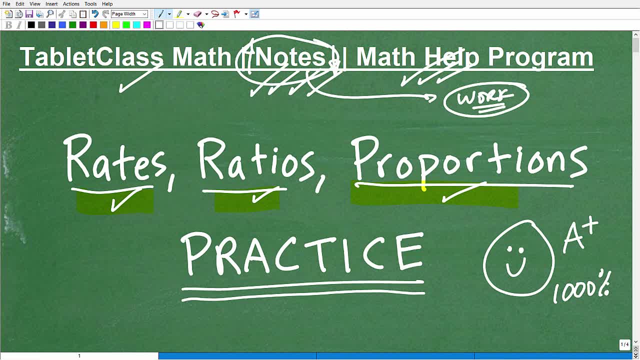 keep it up, because there's a lot of topics that are coming your way. They're going to be new and exciting. As far as this video goes, if you found it interesting or if you liked it in some way, please consider smashing that like. 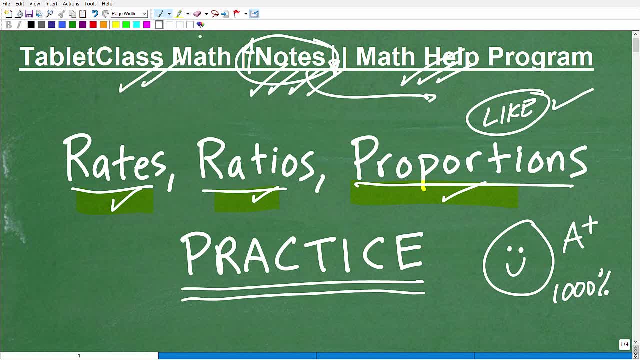 button. If you're new to my YouTube channel, please consider subscribing Again. I've been on YouTube for a long time, 10 plus years. Great platform from someone like myself who's obsessed teaching math in a clear and understandable way. If you really want my best help, check out the resources by. 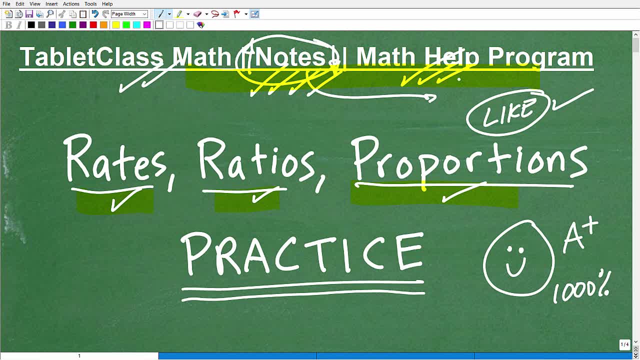 following those links in the description of this video. With that being said, I definitely wish you all the best in your mathematics adventures. Thank you for your time and have a great day. Captions by GetTranscribedcom. Hi, this is Presh Talakar. Quadratic equations are extremely important in mathematics, but unfortunately they can also be very confusing. In this video, I'm going to present a visual and geometric proof so that you understand the quadratic formula intuitively. Imagine you want to solve: x squared plus 2x minus 15 equals zero. You could solve this by graphing the equation x squared plus 2x minus 15.. The points at which the graph crosses the x-axis are the solutions. You could also solve this equation by factoring into linear terms. If you set these linear terms equal to zero, you'll get the same solutions as written in the graph. When those methods don't work, the quadratic formula will always tell you how you can solve any quadratic equation with arbitrary constants a, b and c. So this is a very useful formula, but unfortunately it's not often. presented in an intuitive way. Why exactly does it work? So let's try and understand this geometrically. Let's solve this equation. First, we'll add 15 to both sides, so that we have x squared plus 2x equals 15.. I'll now color code each term. which has a side length of 2 and another side length of x. The area of this rectangle is equal to 2x. Finally, the term 15. I'll represent by a rectangle which has an area of 15.. It doesn't matter what the exact side lengths are. It only matters that the area is 15, so I'm not going to write in the side lengths. But the task we have is: we want to have the two shapes on the left. we want their areas to be equal to the area of 15,. which is the shape on the right. So how can we do that? Well, the first thing we want to do is we want to combine the two shapes And, lucky for us, we have one common side of x, So we can combine these two shapes on one common side. But there's a trick we're going to use. We're going to split the rectangle of 2x into two small rectangles, which are x by 1. And now we're going to join these strips onto each side of the square. So now we have a shape that's almost equal to a square. So what we need to do is we want to add on the little area so that we get a square. So we put an orange rectangle here and each of its side lengths is equal to the area of 15. This is equal to 1.. And so this area is equal to 1.. And in order to balance the equation, we want to add the same area to the right hand side. So what we've done geometrically will represent algebraically, by adding a term of 1 to each the left and the right hand sides of the equation. And this is what's known as completing the square. You've probably heard the term algebra class, but this is the geometric reason. We're literally adding a term to this area so that we can complete a square. And now this helps us solve the problem, because what we want to do we'll simplify that: 15 plus 1 is equal to 16, is, we have a square with the side length of x plus 1 and we need that square to be equal to the square on the right hand side. So we want x plus 1 squared to have an area of 16.. Now, one way we could do this to have an area of 16, is we could imagine having a square that has a side length of 4.. So, in order for our square on the left to be equal to the square on the right, we want x plus 1 to be equal to 4.. We can easily solve this: that x is equal to 3.. But there's another way we can solve this. We can easily solve this: that x is equal to 3.. But there's another way we can solve this: that x is equal to 3.. But there's another way we can solve this. It's kind of an unusual way, but imagine we had side lengths of negative 4. If we multiply negative 4 by itself, we also get an area of 16. So we could also set x plus 1 equal to negative 4.. And that gives us our other solution of x equals negative 5.. So this is the visual way to understand quadratic equations And if you understood this, I'm going to show you this proof, just in a more general way, which is how we get the quadratic formula. So we have a general quadratic equation And the first thing I'm going to do is I'm going to subtract c from both sides, So we have ax squared plus bx equals negative c. We'll now divide by the constant term of a, So we have x squared plus b over ax equals negative c. So we have x squared plus b over ax equals negative c over a. This is very similar to the equation we just solved. It has x squared plus something times x equals a constant term. So let's use the same procedure. We'll represent x squared as being the area of an of a square with the side length of x.